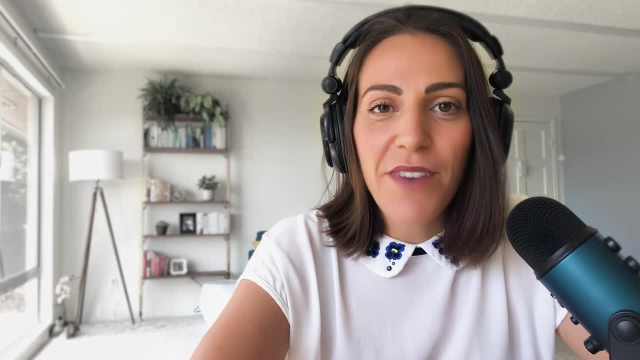 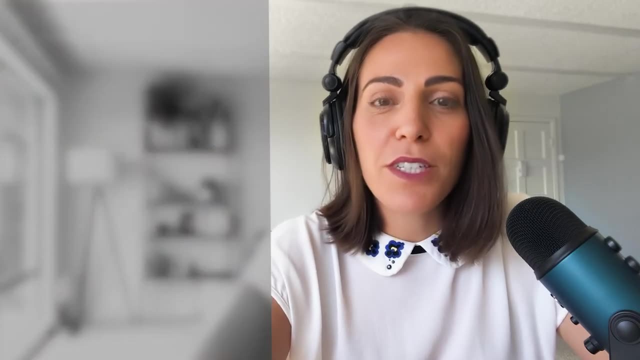 subscribe. Today I'm going to go over the Customer Satisfaction Score, also known as CSAT, which is one of the most popular customer loyalty metrics. First I'm going to explain to you why CSAT is important, then I'm going to explain to you how to calculate it, and then I'll go over how to use. 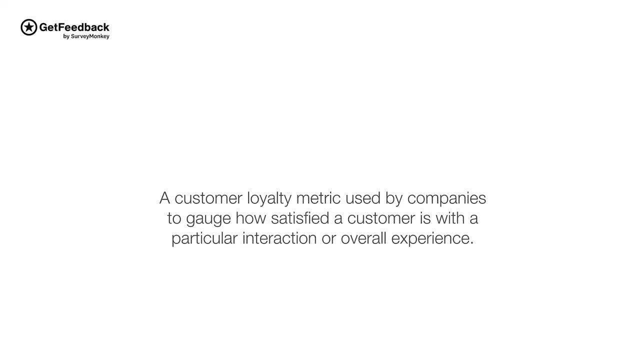 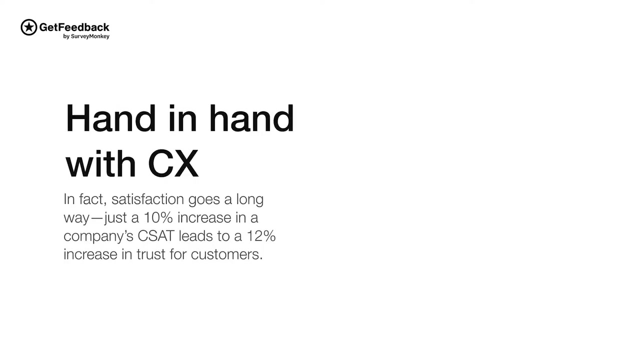 this metric in your customer experience program. CSAT is a customer loyalty metric used by companies to gauge how satisfied a customer is with a popular interaction or overall experience. This metric goes hand-in-hand with great customer experience. In fact, satisfaction goes a long way. 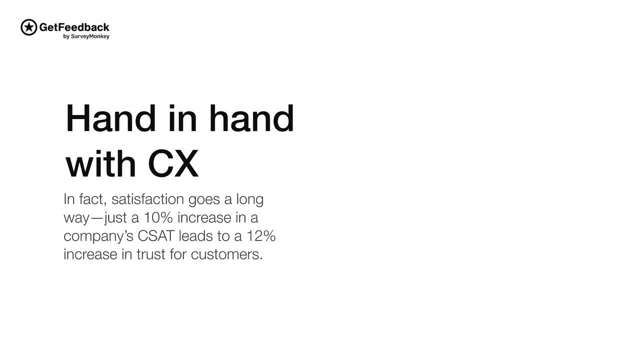 Just a 10% increase in a company's CSAT score could lead to a 12% increase in trust from customers. If you're new to this channel, please subscribe to this channel and hit the bell so you don't miss any future videos. Also, satisfied customers are more likely to upgrade or add. 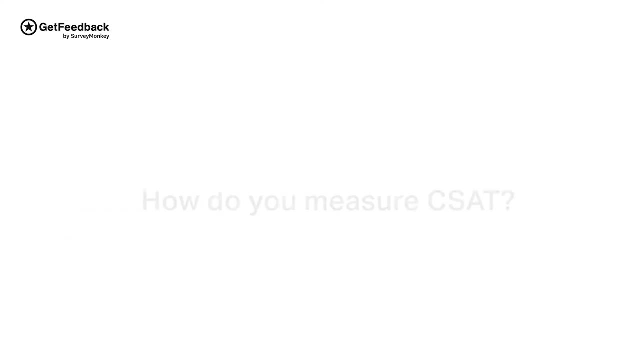 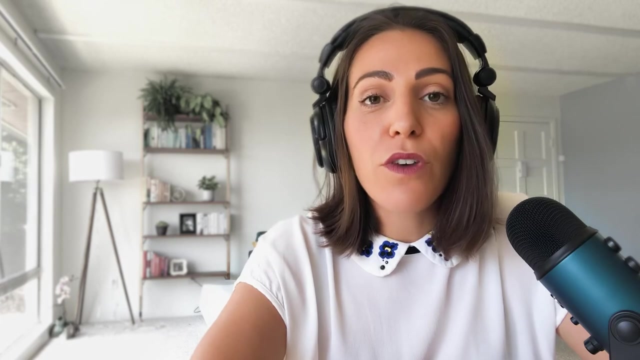 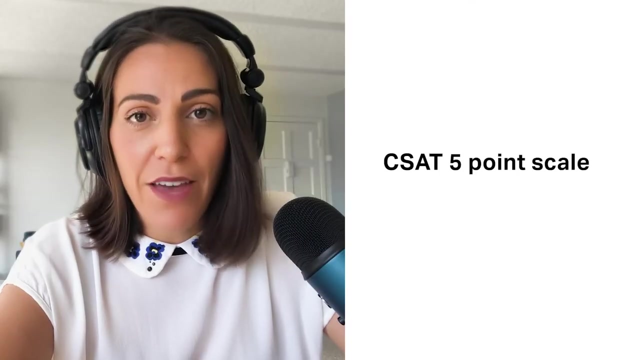 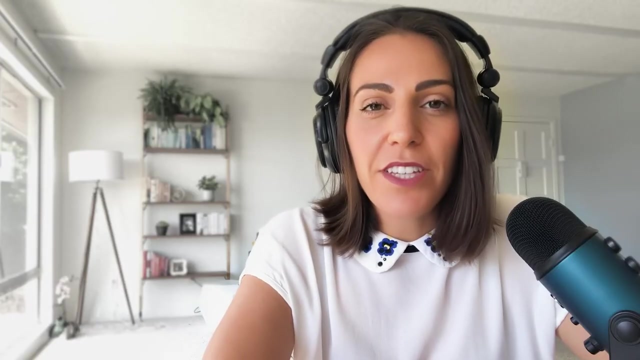 services and are less likely to cancel them. Okay, so how do you measure CSAT? The Customer Satisfaction Score is assessed by asking customers to rate their overall satisfaction with a specific product, service or specific interaction using a five-point scale, one being very unsatisfied and five being very satisfied. The metric is looking specifically: 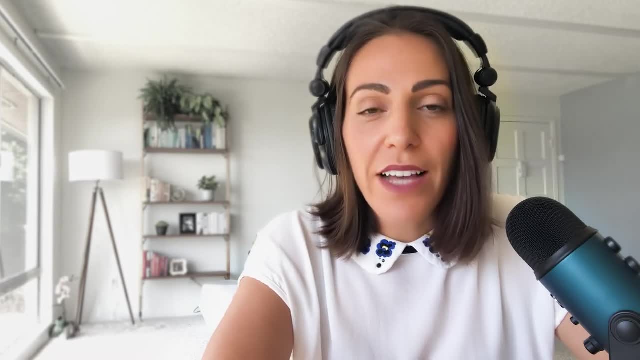 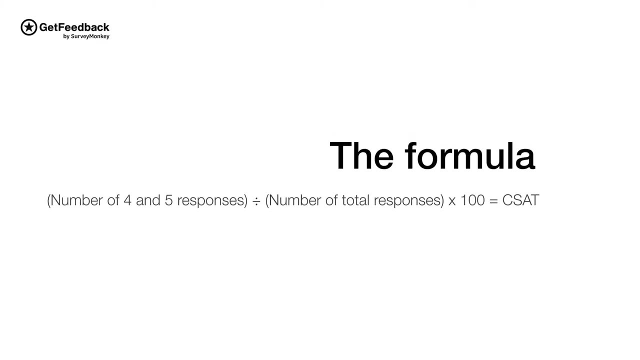 at the percentage of happy customers, which is why, when you calculate the CSAT score, you only take into consideration the four to five ratings. You calculate the CSAT percentage by adding up the total numbers of four and five responses, dividing that by the total number of. 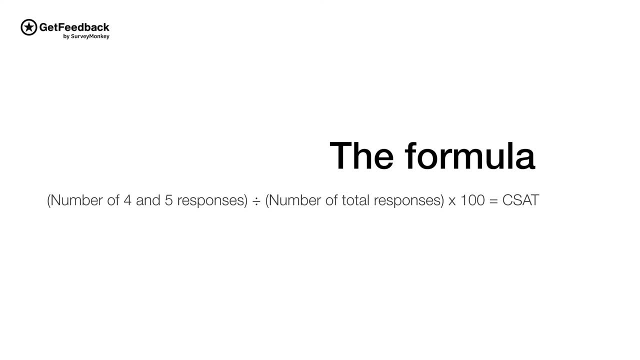 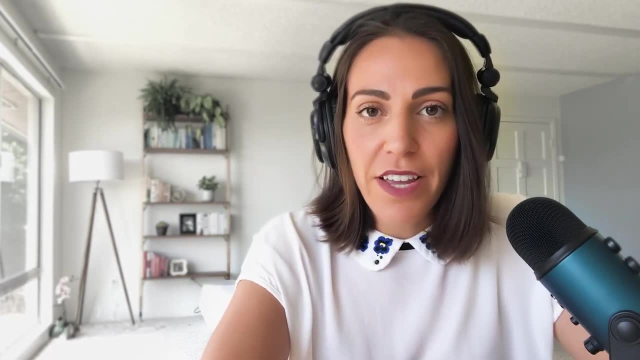 responses and then multiplying that by a hundred. So, for example, if you have a CSAT score of 80%, that means that 80% of the customers who responded to your survey are very satisfied. If you're using CSAT already and you're not sure how you compare it to your peers. 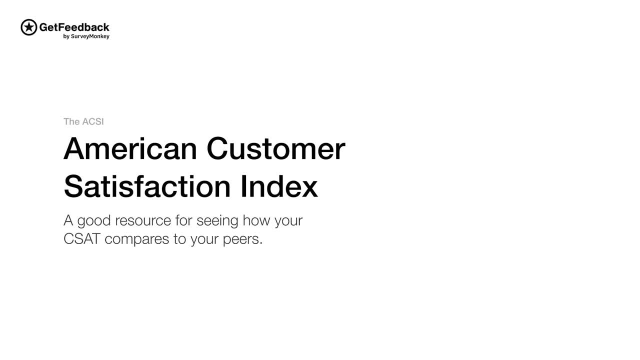 a good resource is the American Customer Satisfaction Index. According to the index, the current overall US Customer Satisfaction Score is 76.5%, But keep in mind that the benchmark will vary by industry, so I recommend going onto their website for the latest information. Customer Satisfaction Score is both a relationship metric and a touchpoint. 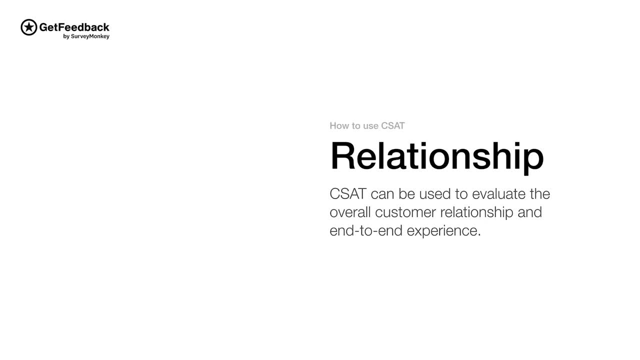 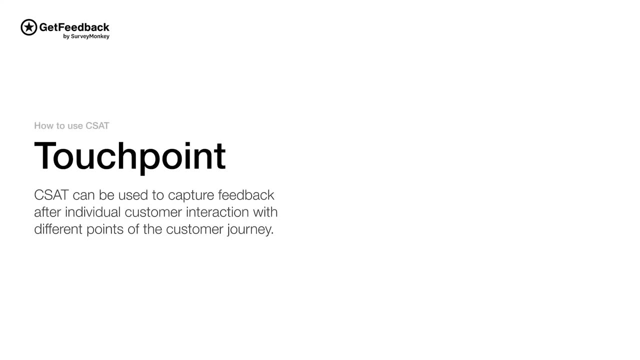 metric. It's a relationship metric in the sense that it can be used to measure customer satisfaction, it can be used to evaluate the overall customer relationship and end-to-end experience And, as a touchpoint metric, it can be used to capture feedback after individual customer.